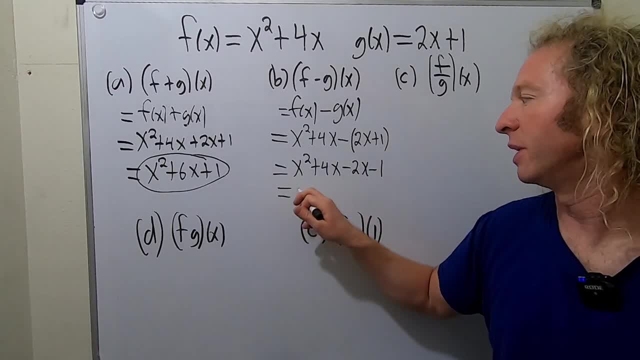 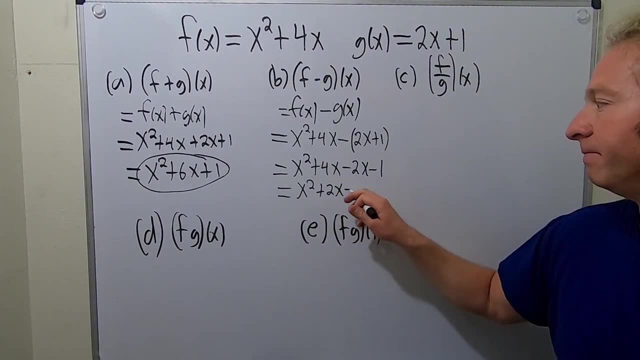 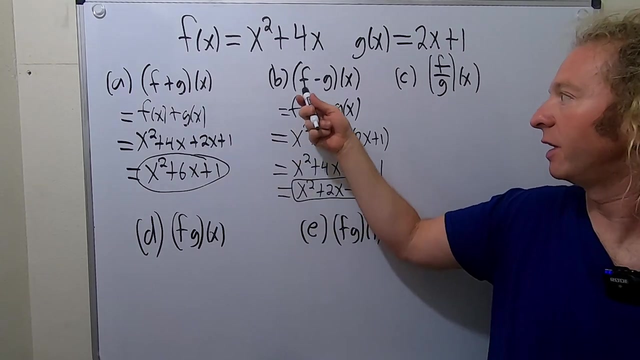 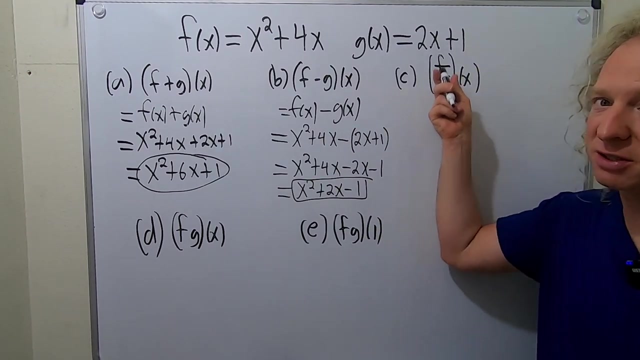 So minus 2x, minus 1.. This will be x squared 4x minus 2x is 2x, And then we have our minus 1.. That's it. So, again, just like before, like here, we replaced f with f and g with g and we put a plus. Same thing here, Right, F with f, G with g, We put a minus, And then, just carefully, be careful, Right, Super careful, This one's much easier- Same thing- Replace f with f and g with g. So this is f of x. 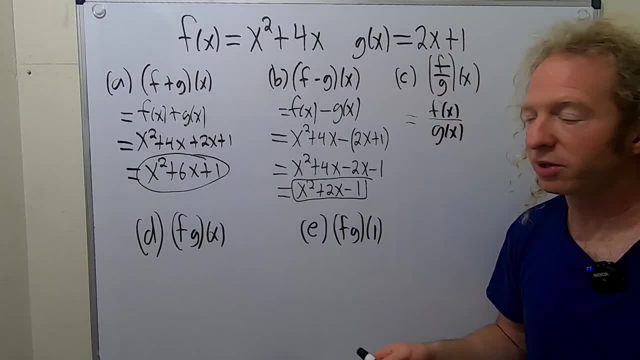 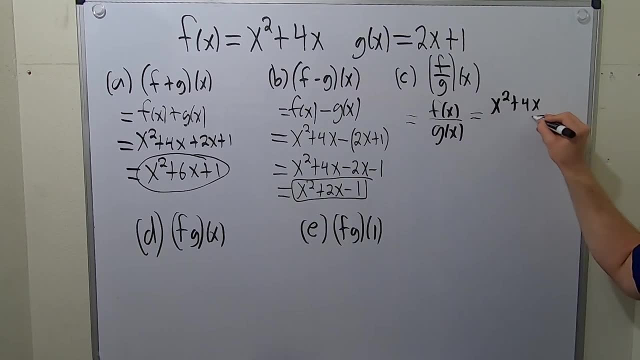 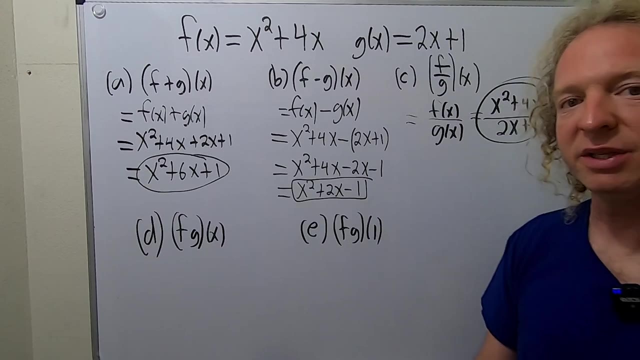 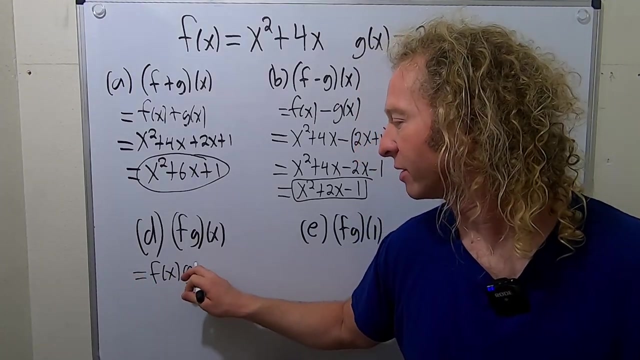 Right. F with f and g with g Always works. And then now just replace f with what it is. F is x squared plus 4x, So x squared plus 4x, And then g is 2x plus 1.. So 2x plus 1.. Very good, Awesome, Pretty easy. Same thing here, Right? Except this time it's times, Right? So it'll be f of x times g of x- A little bit more annoying because we do have some work to do. So f of x is x squared plus 4x. 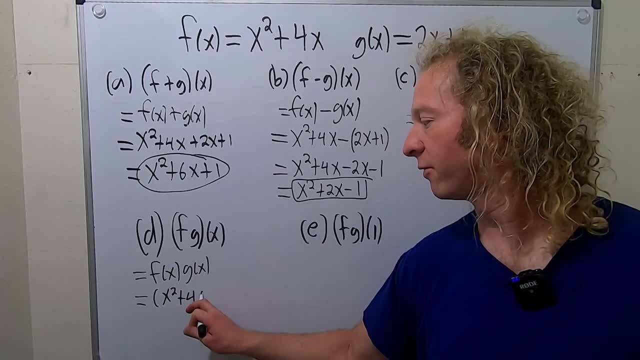 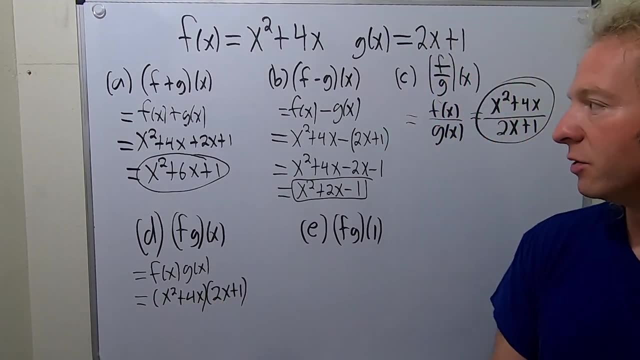 So it'll be x squared plus 4x- Good stuff. g of x is 2x plus 1.. Right, So this will be 2x plus 1.. So they're all the same, really. You just basically have different operations. So now we have to distribute. 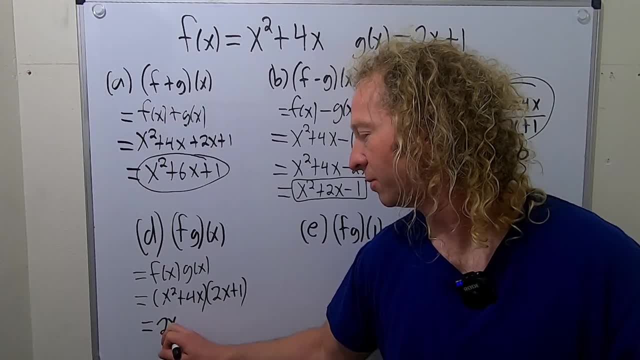 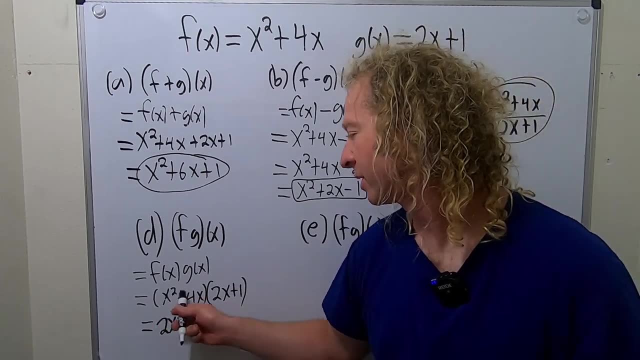 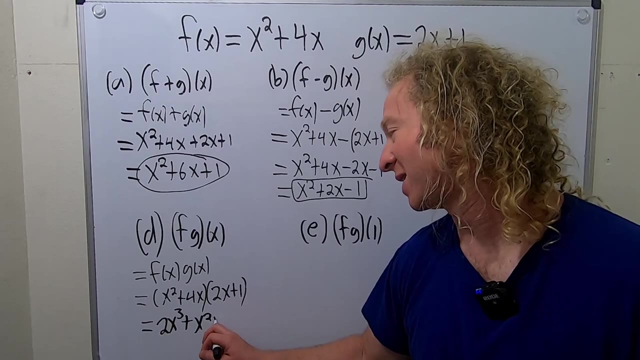 So x squared times 2x is 2x cubed And x squared times 1 is x squared Right. So this times, this is this, This times, this is this: Now you distribute to 4x Times 2x is 8x squared. Almost messed up. 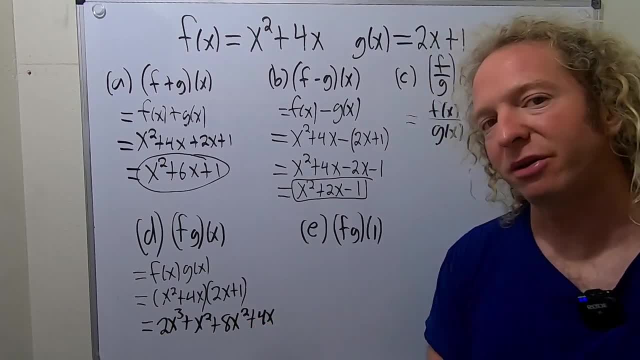 4x times 1 is 4x. Let me go over that again just to make sure that I did it right. So x squared times 2x is 2x cubed x squared times 1 is x squared Good. 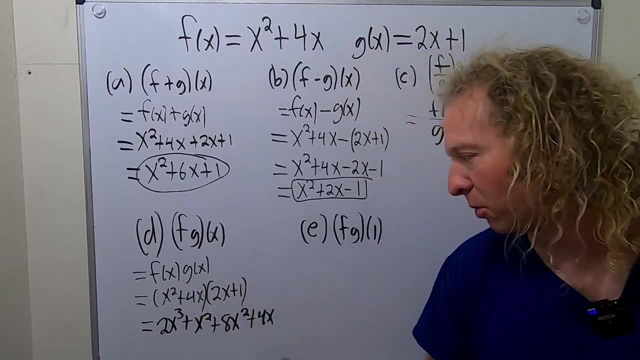 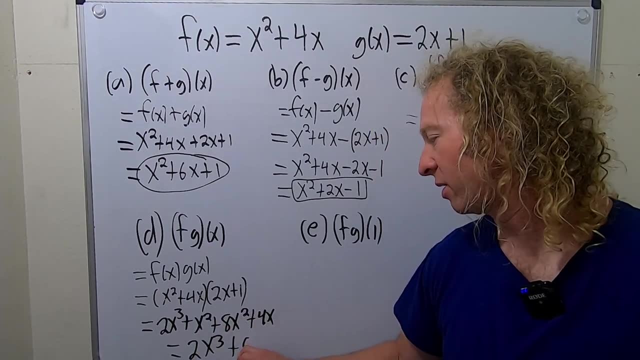 4x times 2x is 8x squared. 4x times 1 is 4x Boom, We got this And this is equal to 2x cubed x squared, plus 8x squared is 9x squared. 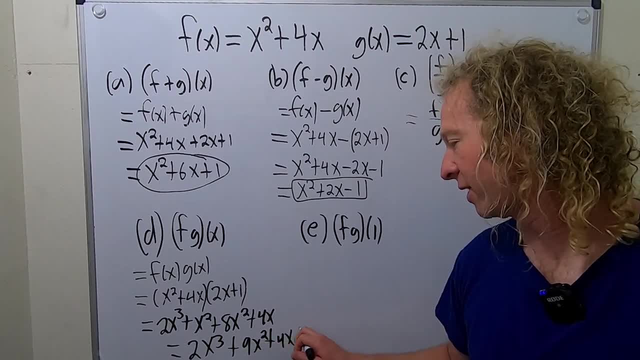 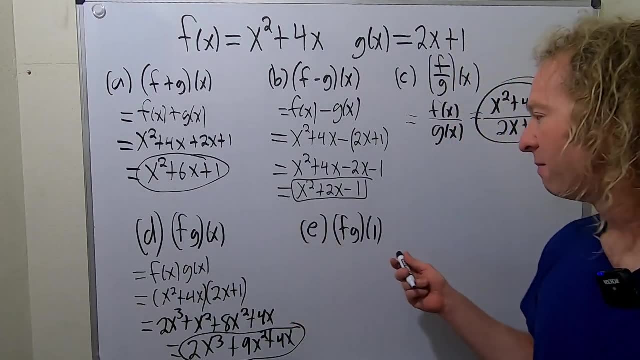 And then we still have the 4x Beautiful stuff. That is, the multiplication of functions. The last one's really easy and I kind of threw it in because a lot of times you see this: Basically you just plug in 1 to the answer you got here, Right?